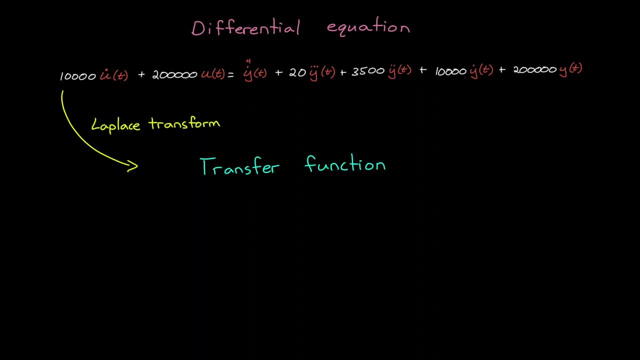 time. We can convert it to a transfer function using the Laplace transform, and I'm not going to cover the Laplace transform in this video, but if you'd like to learn about it, I've left some links below. But for linear differential equations like this, it's enough. 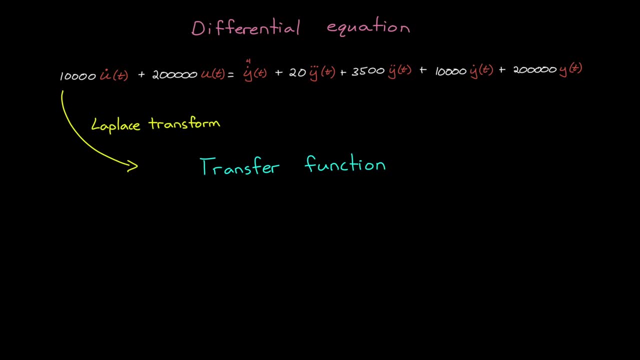 to know that derivatives, with respect to time, turn into exponents of the complex variable s. So y of t, which isn't a derivative, becomes s to the zero times y of s, And y dot of t, which is a derivative, would become s to the one times y of s, since it's a single derivative. 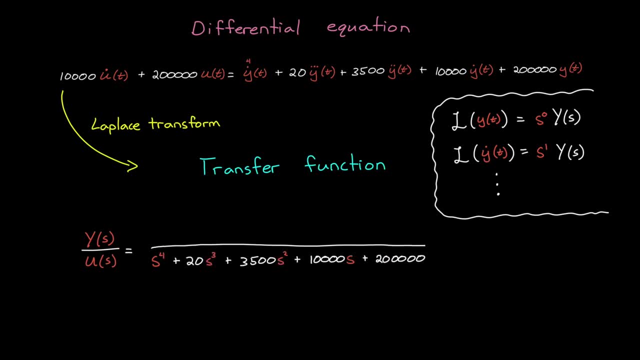 And using this logic, we can transform the differential equation in the time domain into an equivalent transfer function in the complex plane or the s-domain. These two models capture the same system dynamics. However, with a transfer function, we describe the system as a function of s instead of a function of time, And s is a complex variable. 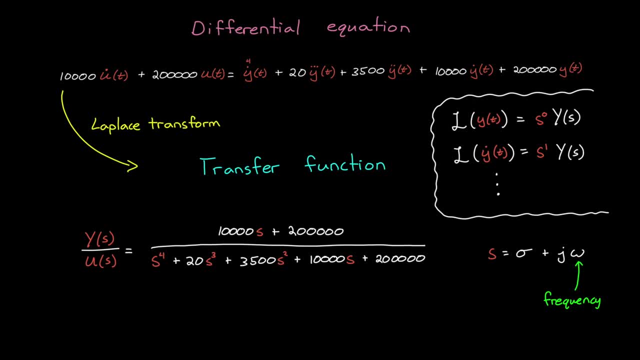 sigma plus j, omega, where omega relates to the frequency of a signal and sigma relates to the exponential growth or decay of a signal. So if we have the input as a function of s or we describe the bump in the road in terms of frequency and exponentials, then we can transfer it through the 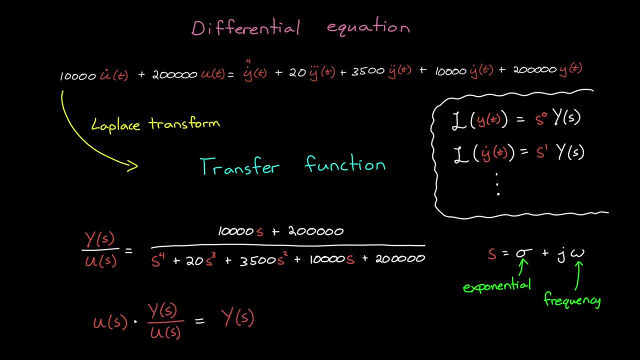 system by multiplying it with the transfer function. In this way, the transfer function is the ratio of the output over the input in the s-domain. Okay, so this is good and all, but why would we choose to model a system in this strange form instead of a differential equation? Well, 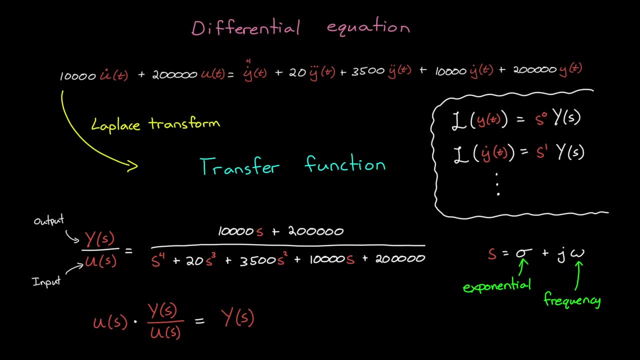 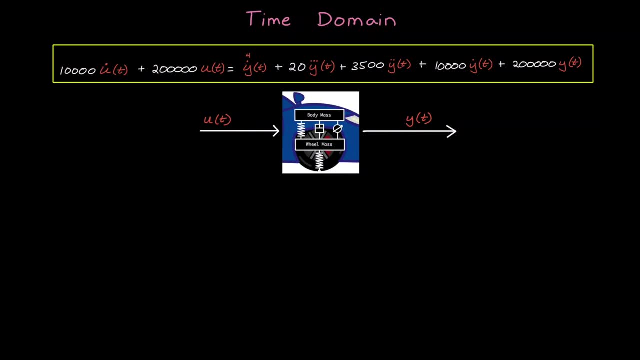 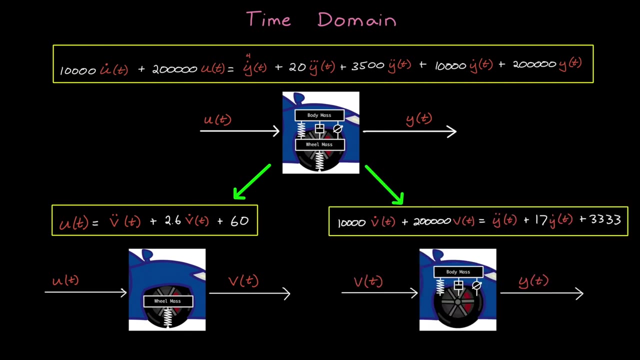 for one. differential equations don't do well in series. Imagine this: Instead of an end-to-end model of the suspension system with a single differential equation, what if we had one differential equation that modeled just the tires and then another differential equation to model the shocks and the springs? So the output v of t of the first. 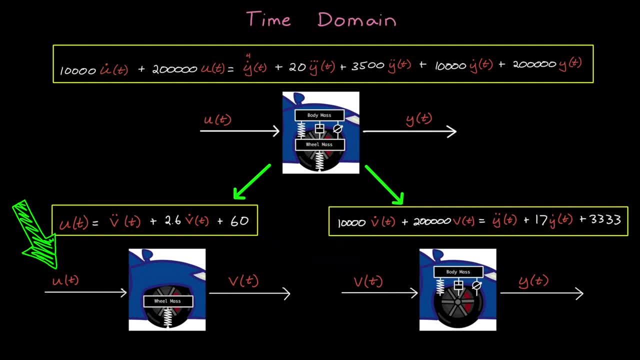 equation is the input to the second, And if we wanted to see how an input u affects the motion of the car y, we would have to solve for the response of the first differential equation, v, and then convolve it with the impulse response of the second differential equation. 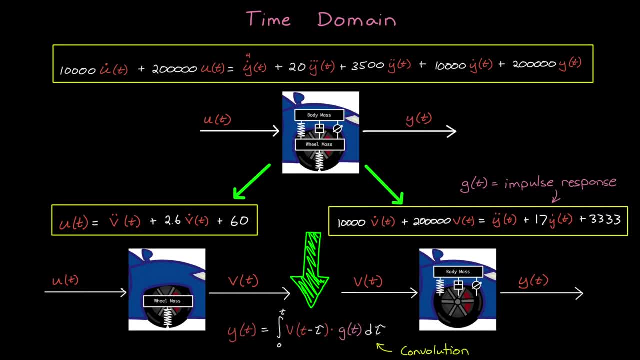 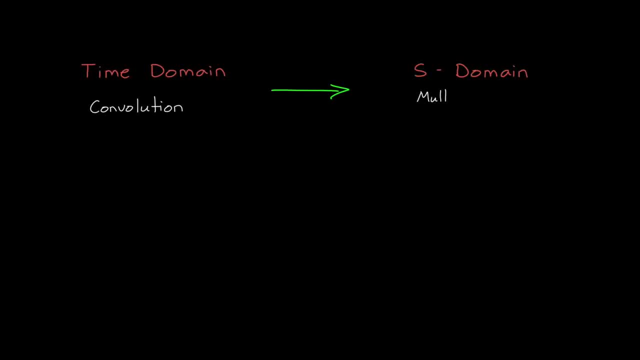 which I'm calling g, And the convolution integral is a rather math-heavy operation. On the other hand, convolution in the time domain becomes multiplication in the s-domain. Therefore, to combine the equivalent two transfer functions in series, we just have to multiply them And I think we can agree that polynomial multiplication. 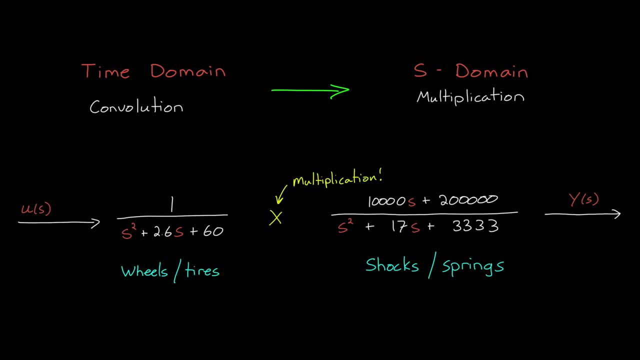 is easier than convolution. So in this way transfer functions are nicely suited for block diagram representations, since combining blocks is as easy as multiplying them. But there are other good examples of transfer functions in the s-domain. There are other good reasons to choose a transfer function to model your system. 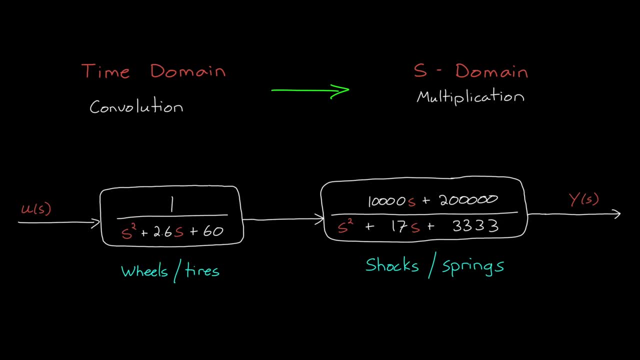 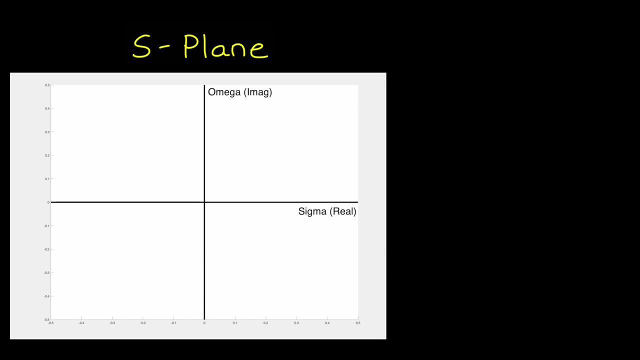 And one is that we get different insights into the system by looking at the s-domain instead of just the time domain. Remember, s is a complex variable that consists of the real component, sigma and the imaginary component, omega, So all of the values of s can be displayed. 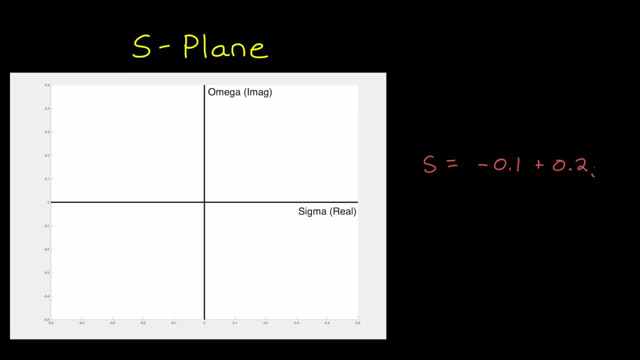 on a 2D plane. So, for example, s equals minus 0.1 plus 0.2j would be right here. Now a transfer function is a function of s, So we can calculate the value of this function s over s plus 0.3,. 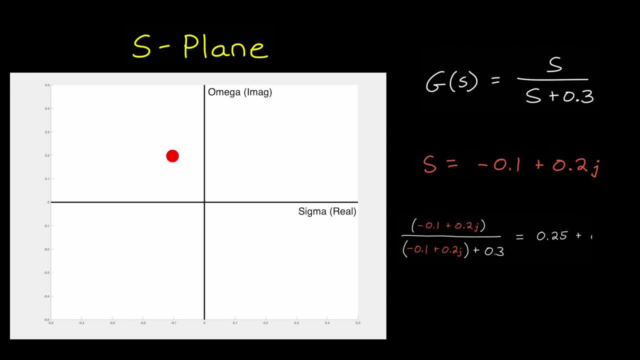 for this value of s. This is analogous to plugging in different values of t in a time domain function. So for s equals minus 0.1 plus 0.2j, this transfer function has the result 0.25 plus 0.75j. 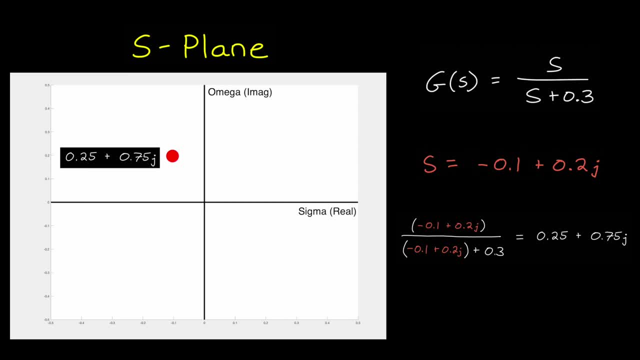 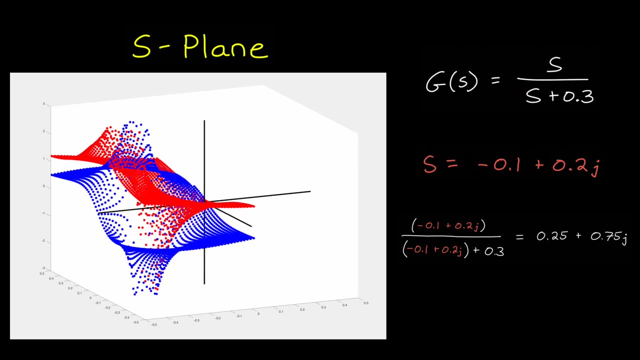 Now, to show you what the entire s-plane looks like for this transfer function, let me rotate the axis so that I can plot the value along the vertical, And now I'm just going to cycle through lots of different s-values across the entire plane. Here the red values are the real component. 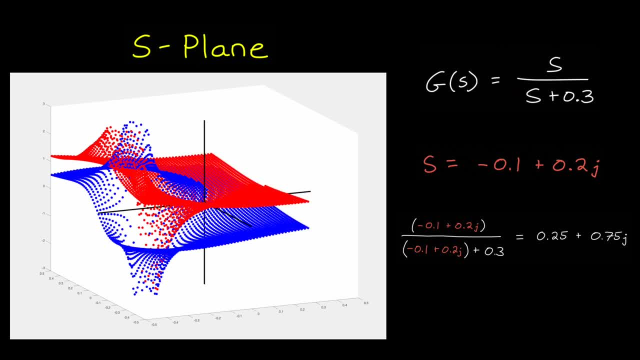 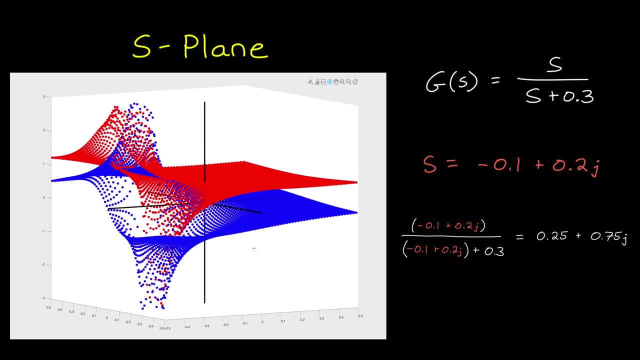 of the result- and blue are the imaginary components- And check this out. We're left with this kind of interesting landscape of peaks and valleys. And just like how we looked at information in the time domain to understand how the system behaves over time, we can now look at 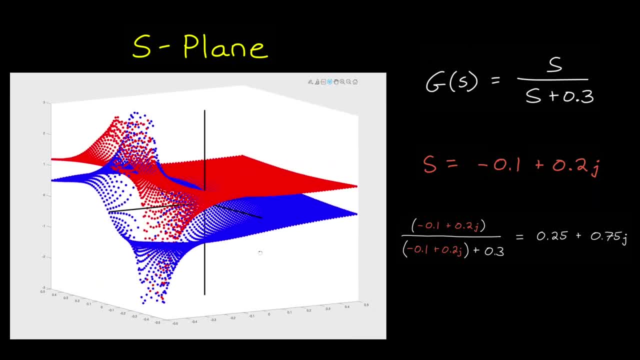 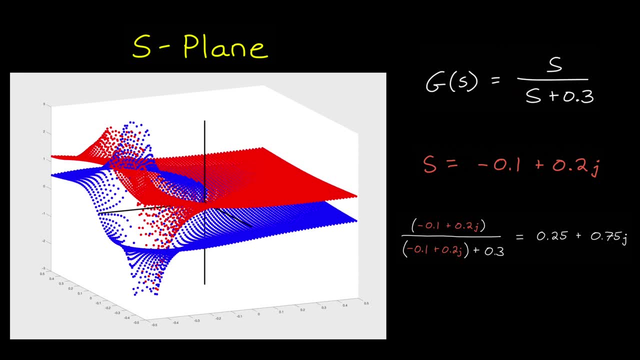 this information To understand how the system behaves over frequency and exponential motion. Of course there's a lot of information here And, I'll be honest, looking at it this way is cumbersome and difficult to interpret, But luckily we don't have to concern ourselves. 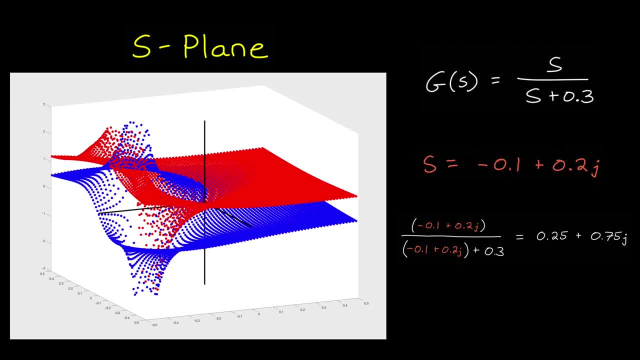 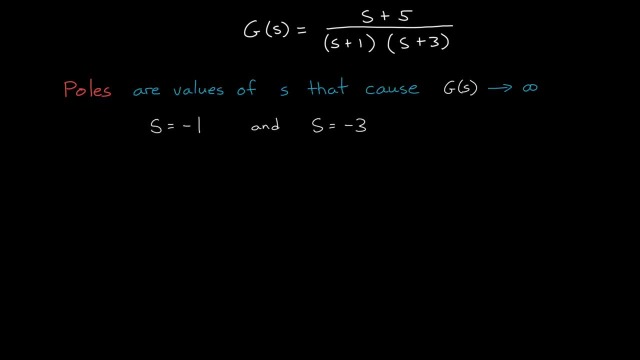 with most of these values, because all of the information in this complex plane is captured by the gain of the transfer function and the locations of the poles and zeros. So let's take a look at some of the values that we need to know about the transfer function. 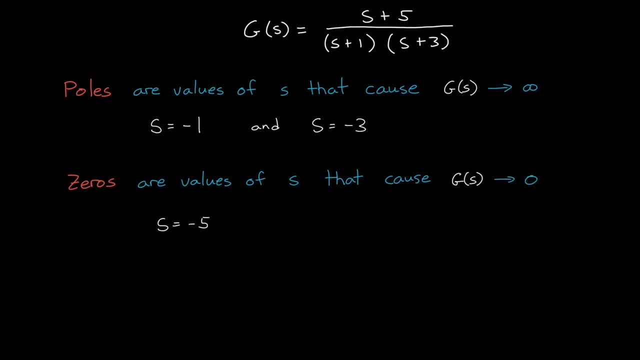 So we have the value of s that causes the function to go to infinity, And zeroes are values of s that cause the function to go to zero. And gain is the ratio of the output and input under steady state conditions Or, more easily, it's the value of the transfer function when you set s to zero. 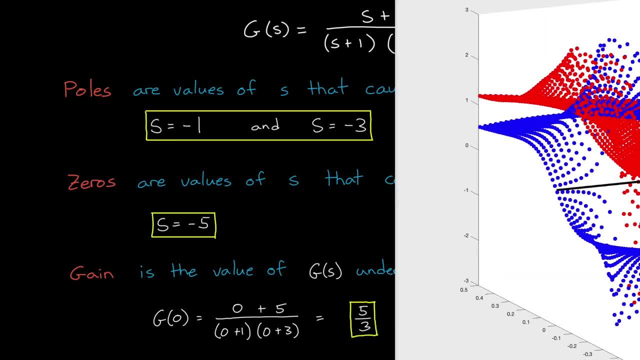 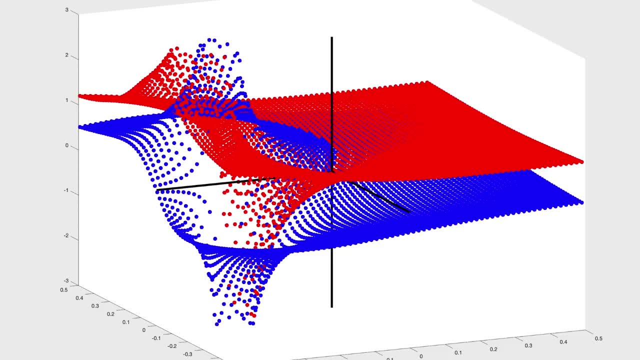 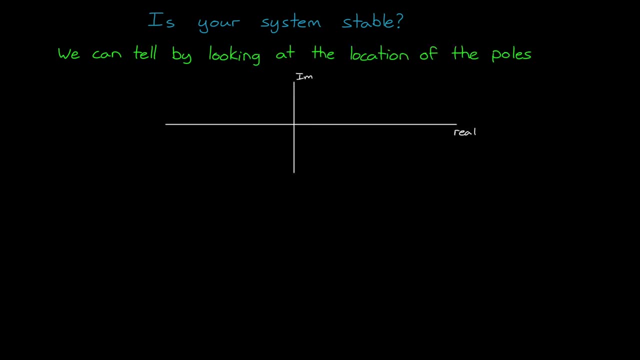 And so we really only need to know these three things- Poles, zeros and gain- And we can understand the entire s-domain. For example, we can use the s-domain to determine if a system is stable by looking at the location of the poles, If any pole is in the right half of the complex plane. 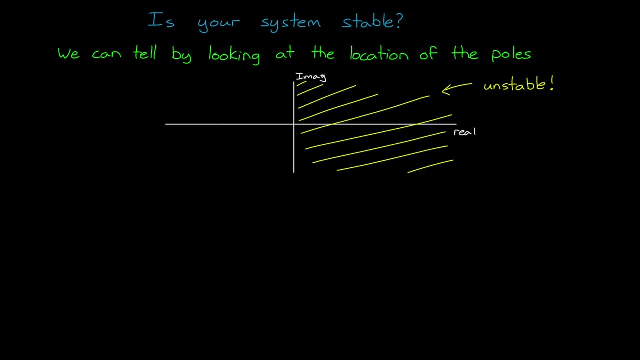 that is, that sigma has a positive value, then the system is unstable. So, for example, this transfer function has a pole at minus 0.3, and so it's stable. And this becomes really powerful when we have transfer functions in series. 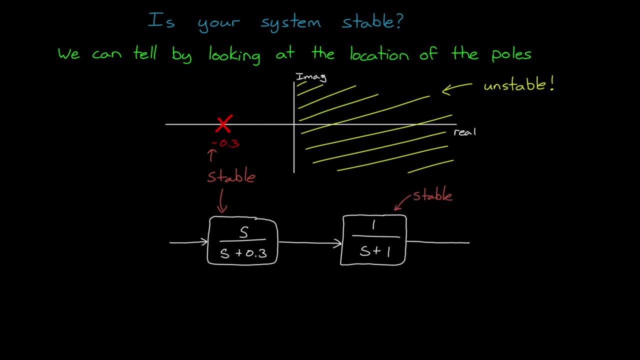 since we combine them together, And that's why we need to know the location of the poles. If any transfer function is unstable, then the end-to-end system is unstable. We can also analyze stability in feedback systems by solving for the closed-loop transfer function and checking the location of the poles. 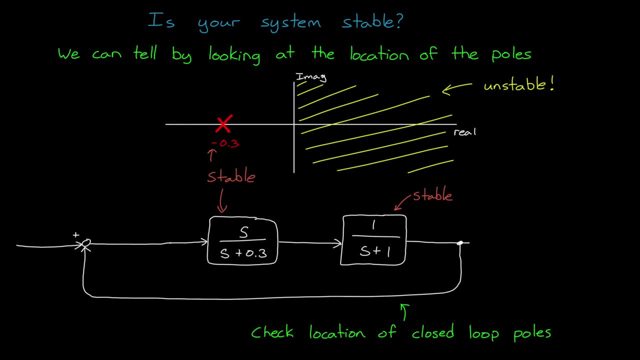 But analyzing a system is just one perk of transfer functions. We can also use them to design systems. specifically when we're concerned with frequency domain characteristics, like we might be with filters and feedback controllers, We can add gain and poles and zeros to our system in such a way as to achieve a desired behavior. 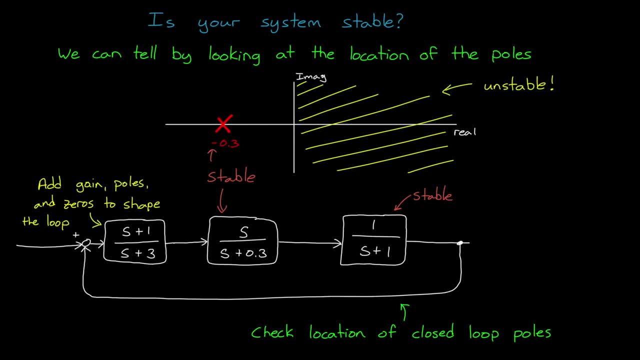 And something that I find really amazing is that we don't even need to find the closed-loop transfer function to determine closed-loop stability. We actually know a lot about the closed-loop system just by looking at the poles and zeros of the open-loop transfer function.